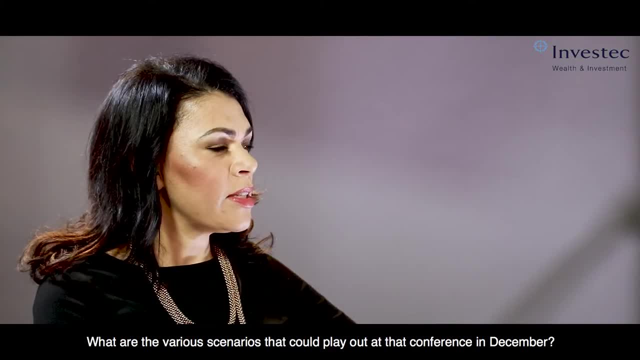 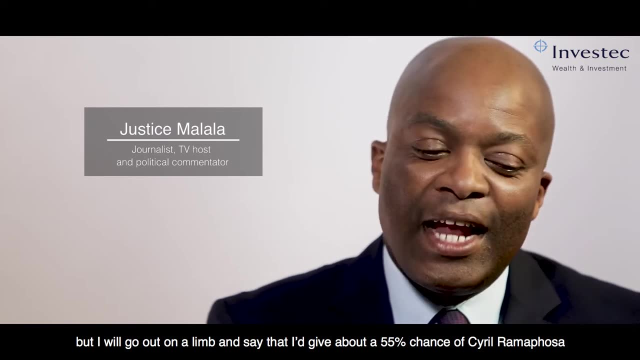 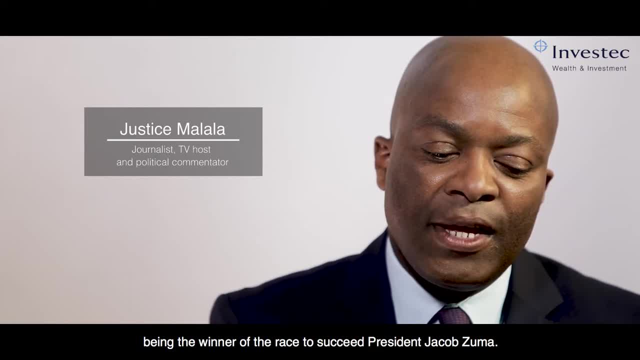 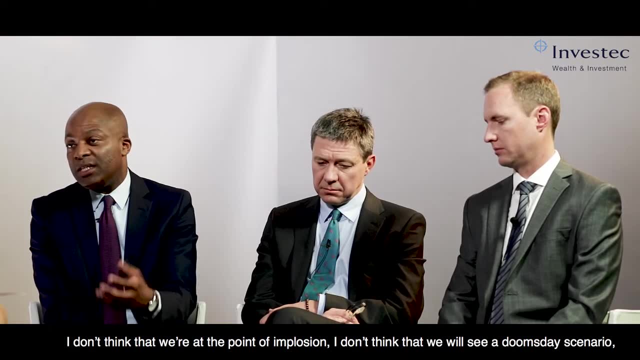 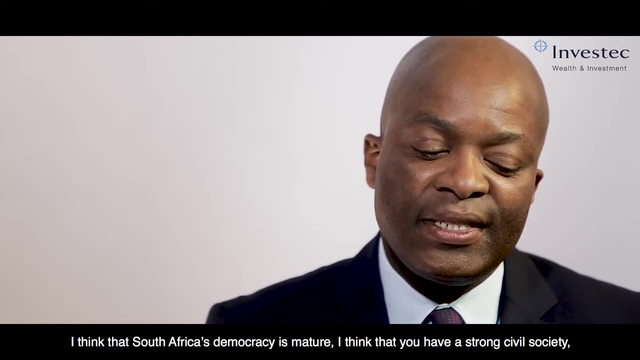 a 55% chance of Cyril Ramaphosa being the winner of the race to succeed President Jacob Zuma. I don't think we're at the point of implosion. I don't think that we will see a doomsday scenario. I think that South Africa's democracy is mature. I think that you have 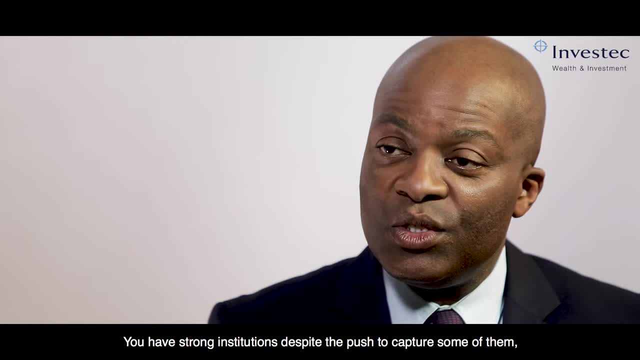 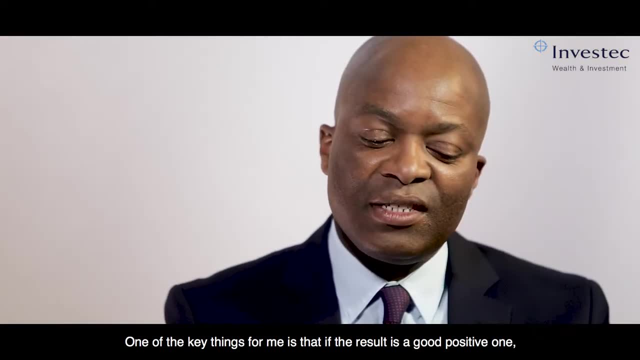 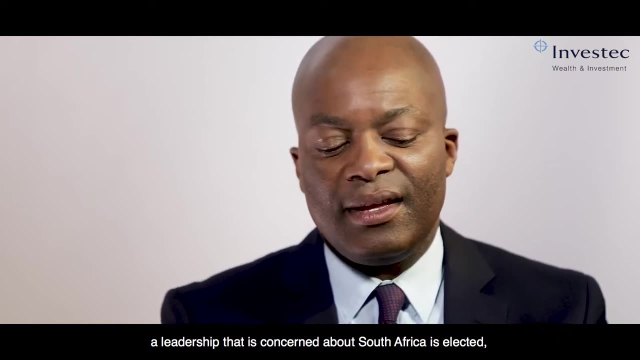 a strong civil society. You have strong institutions. despite the, Despite the push to capture some of them, One of the key things for me is that, if the result is a good, positive one, a leadership that is concerned about South Africa is elected. 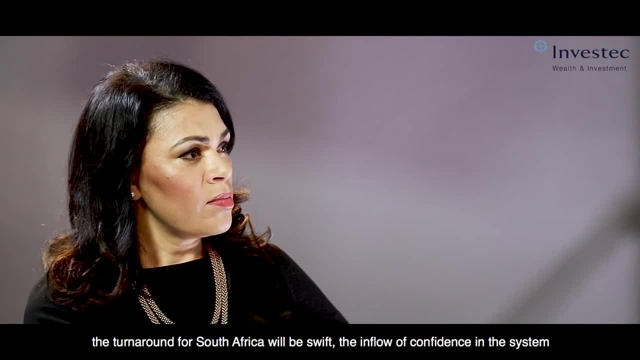 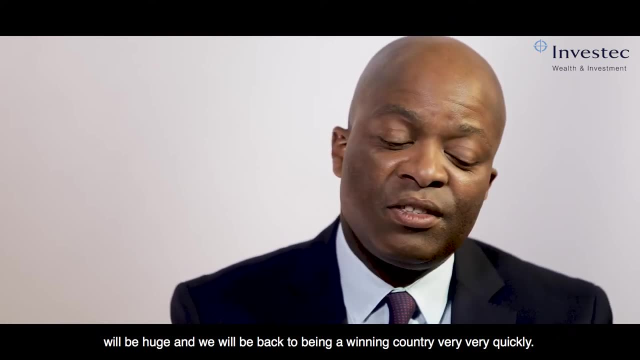 the turnaround for South Africa would be swift. The inflow of confidence in the system would be huge and would be back to being a winning country very, very quickly. I think you're absolutely right. There is pent-up demand for South Africa, So you can. 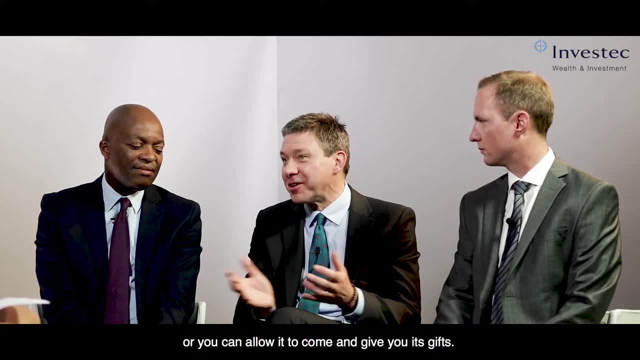 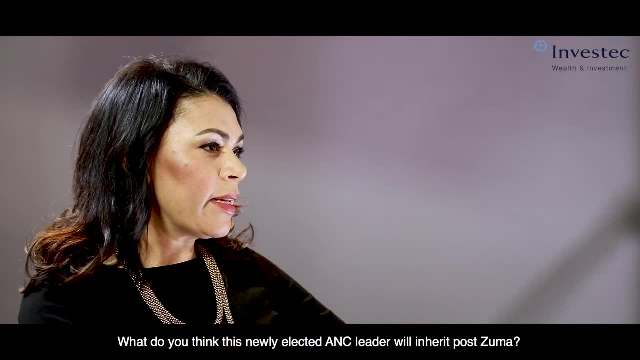 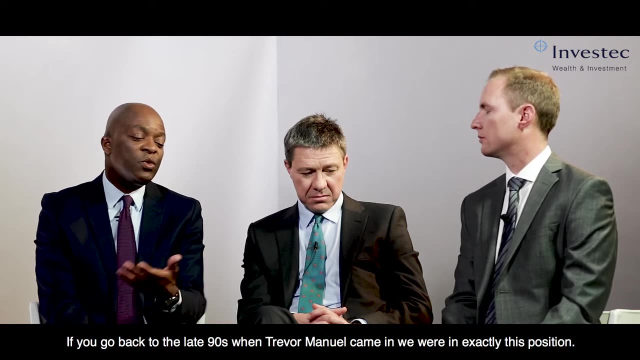 choose to look a gift horse in the mouth, or you can allow it to come and give it its gift. So that's the choices that you're facing. What do you think this newly elected ANC leader will inherit post-Zuma? The government is so lucky that it has a script to work from, If you go back to the late 90s. 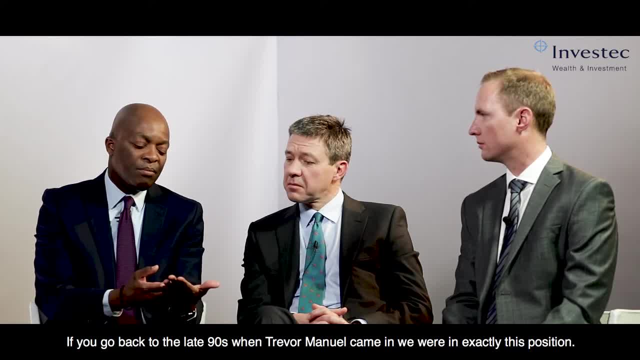 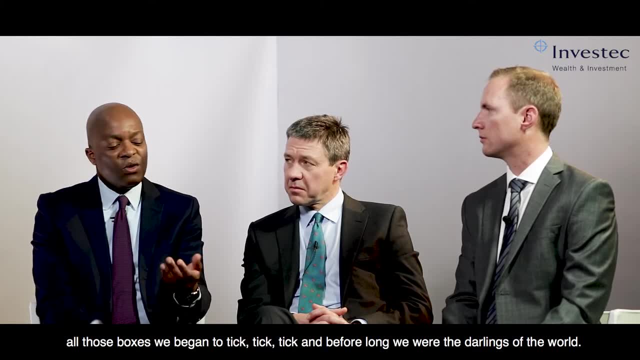 when Trevor Manuel came in, we were in exactly this position: Managed to clean up the finances, made sure that our debt is not spiralling out of control. All those boxes, we began to tick, tick, tick and before long we were the darlings of the world. 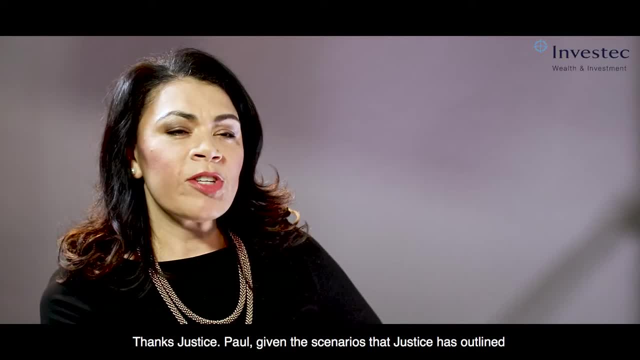 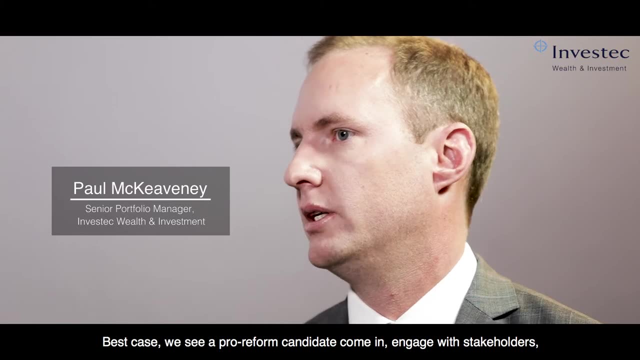 Thanks, Justice. Paul, given the scenarios that Justice has outlined, what are the economic implications? So you know, best case we see a pro-reform candidate come in, engage with stakeholders, address state capture issues, focus on, at least start taking some action on the SOEs. 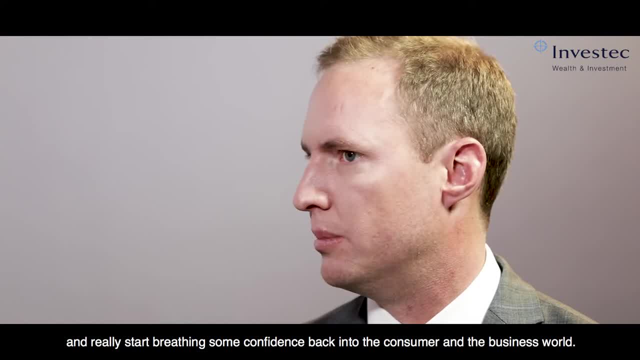 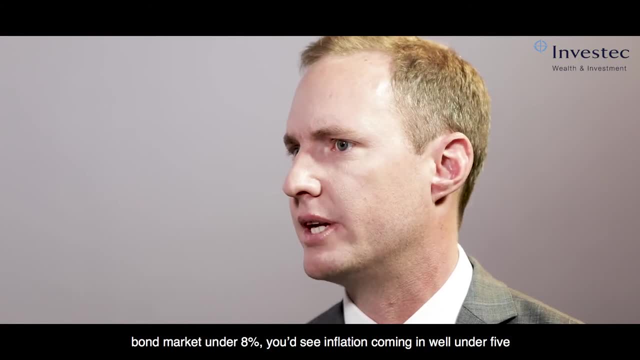 and really start breathing some confidence back into the consumer and the business world. Under this scenario, you'd see- you know- the RAND heading back to 12 quite quickly. bond market under 8%, you'd see inflation coming well in under 5,, all of which would bode very well for the economy.